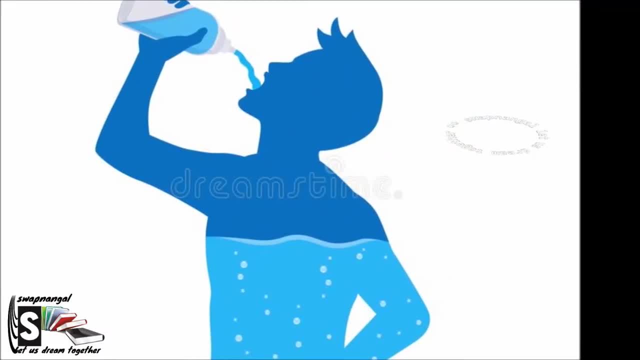 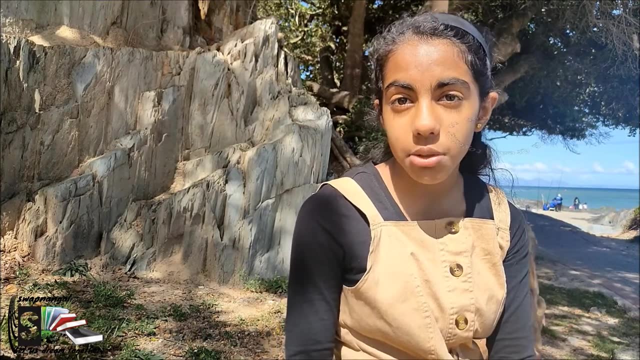 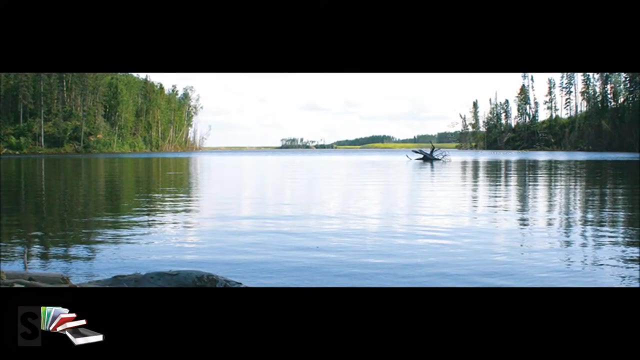 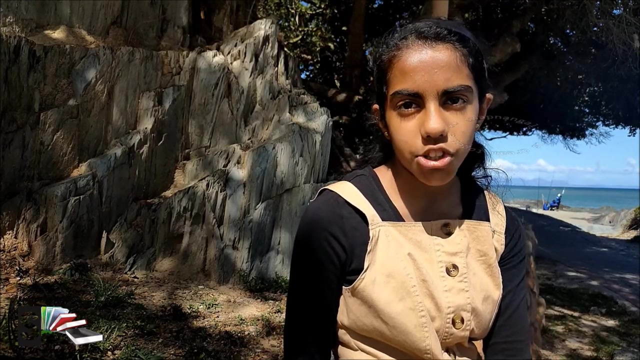 But when it comes to water, A healthy person can survive without water for about three days. again, many factors can change this, like how the person's body uses the water, how much water is needed for the person's body, and we can't survive without water. so we mustn't waste or pollute it, because if we do, we wouldn't have any water to 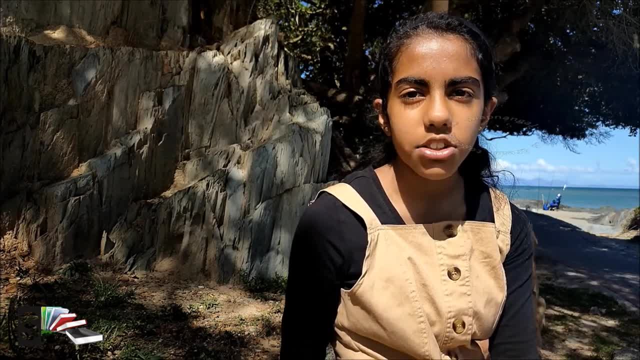 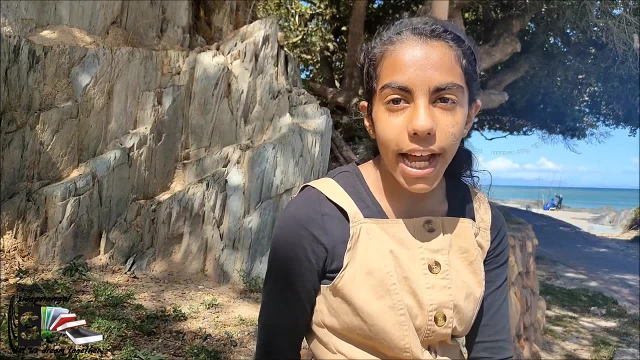 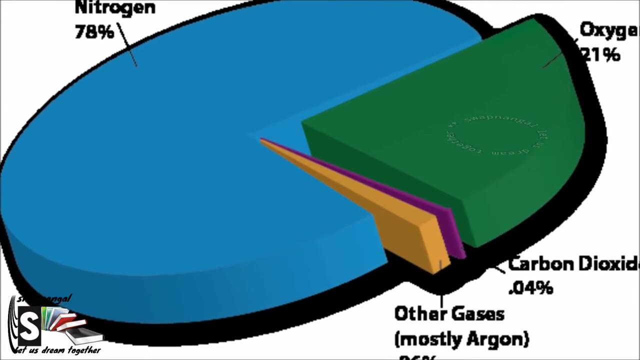 drink and including all the living things on earth. air is another vital natural resource. without air, there would be no life on earth. both plants and animals need air to survive. in the air there are different kinds of gases. oxygen is one of them, and it helps animals and 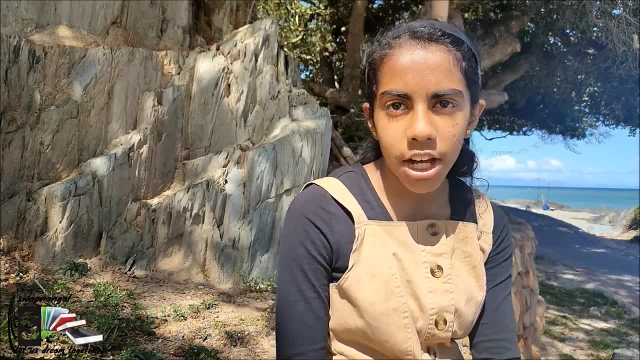 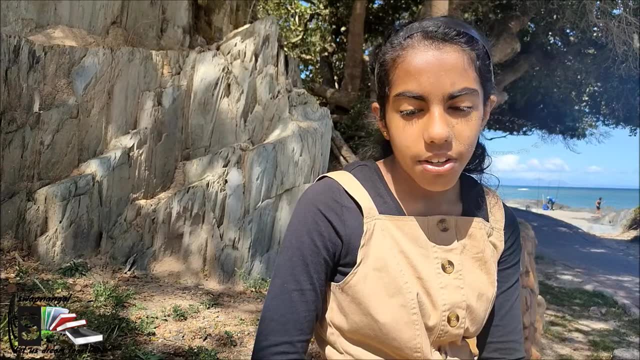 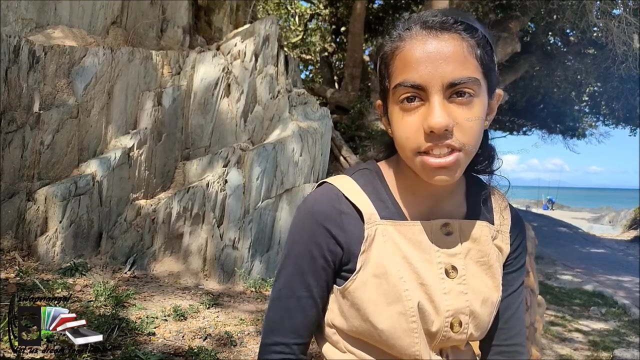 humans to breathe. we breathe in oxygen and breathe out carbon dioxide. carbon dioxide is another gas. it is inhaled by plants. we mustn't pollute the air or harm it, because we need the air, as well as other living things need the air to stay alive. the layer on the surface of the earth where we 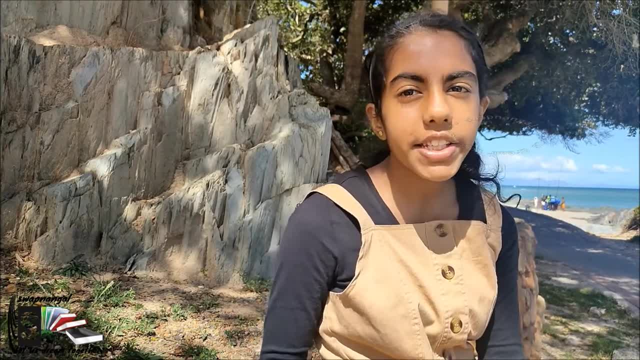 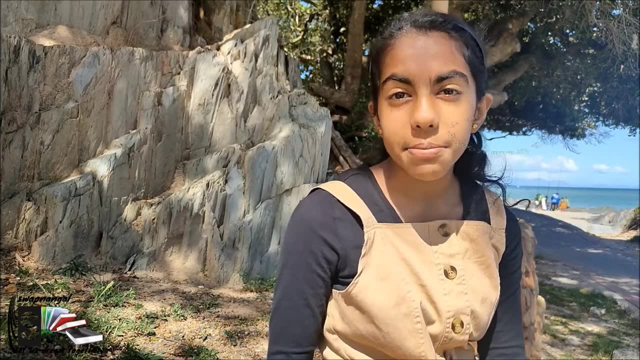 walk and plants grow is called the soil. it is another important natural resource. without soil, there would be no life on earth. the soil is made up of decaying animals, plants and animals. it is made up of decaying animals, plants and animals. it is made up of decaying animals. 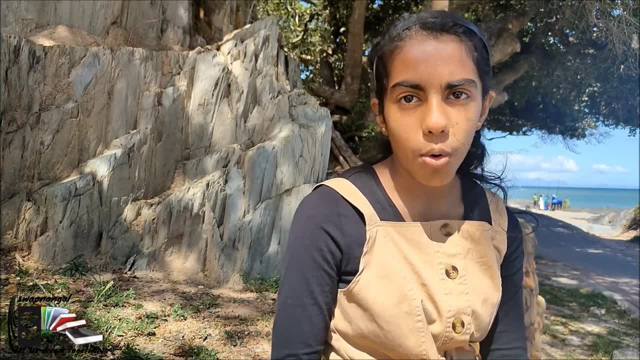 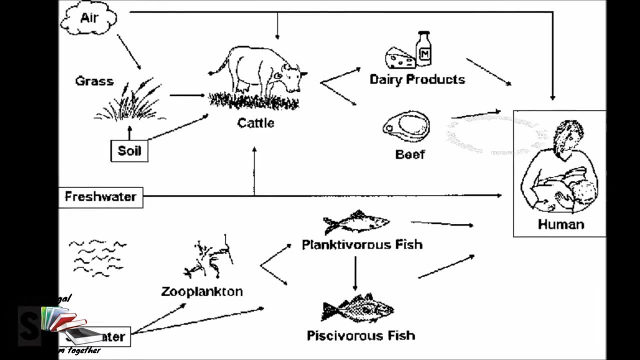 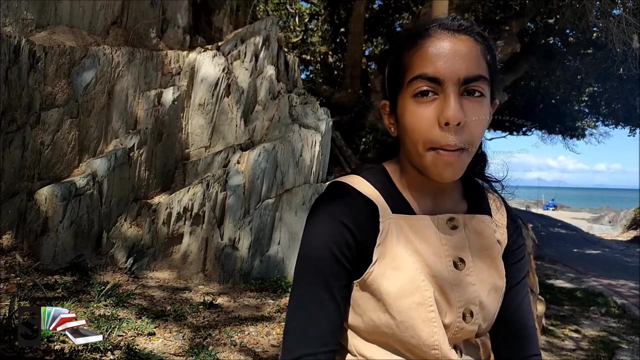 particles of rock plants, air, water and more. the plants grow in the soil, and the plants provide food for us and other animals through a food chain. animals and marine life are a source of food for other animals and for humans, making it another important natural resource we use. 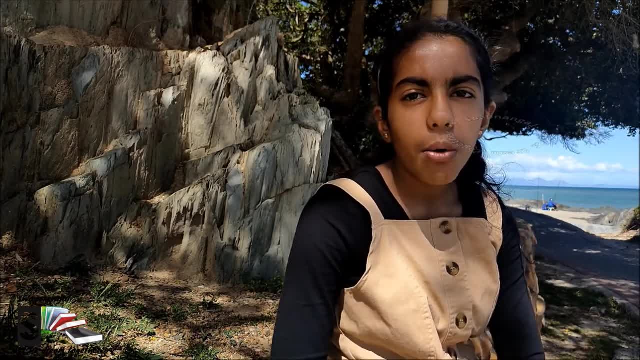 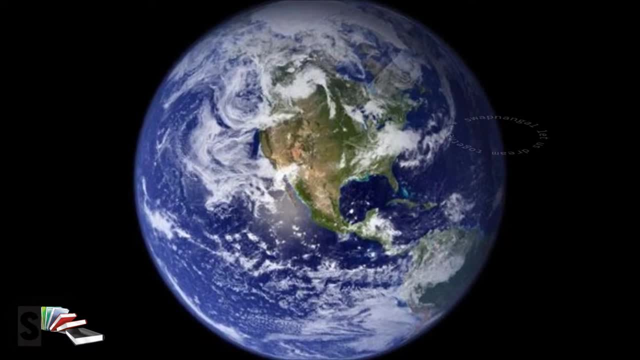 the animals: meat, eggs and milk. we get our protein from the animals, as it is high in protein a the animals: meat, eggs and milk. we get our protein from the animals, as it is high in protein. a million people live on our planet and we all need to use natural resources.